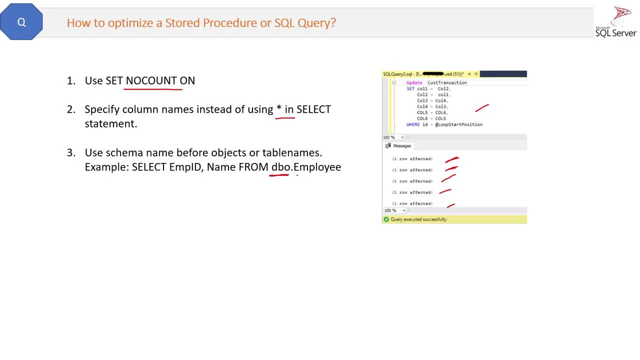 any other schema as per your project. So use it before the table name, because if you have more than one schema, then this query will check in all the schema that where is this table, and that is again not good for performance. Next is: do not use dynamic queries. They are vulnerable to SQL injections. 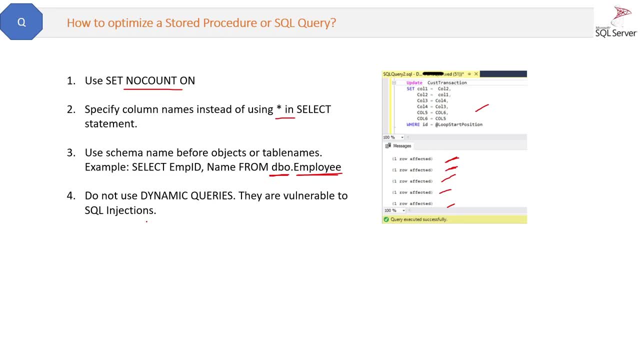 Dynamic queries are runtime queries, I can. this is a different topic, although, but if you know about them, this can be a point. dynamic queries because somebody from the outside can write and insert these dynamic queries in via the SQL injections. next is use exists- you have might have seen like if exists, this statement in. 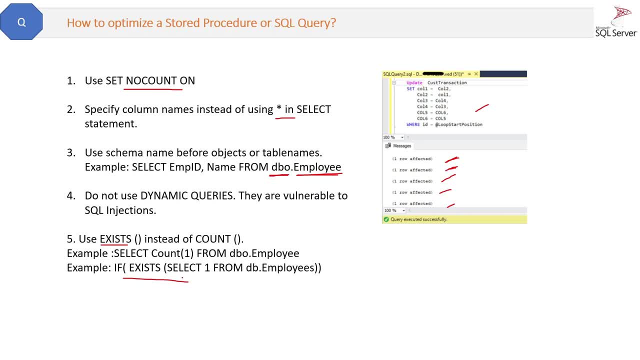 lot of stored procedure. so instead of using count, use if exists. so this is the wrong way. select, count one from DB- your employee and then you will check. rather, use this technique if select one from DB one employees, so use exists instead of count, then use transaction when required only. 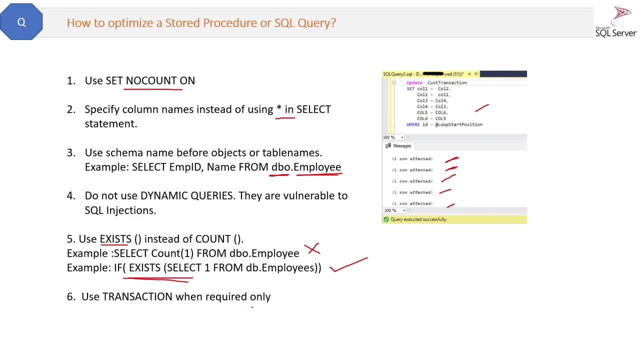 transactions are basically to maintain that all the statements inside the transaction are must execute or none of them execute. so you are, if you are writing a transaction statement and inside this transaction, between the begin and end, if there are three statements, all of these three statement will execute or none of these three statements are executed, that 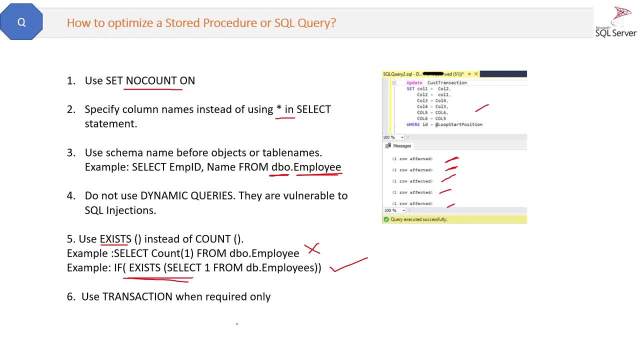 is a good practice, but use them only when required. if it is not required, do not use them in your stored procedure. there are many more things for performance, but I am keeping it short and crisp for now between the two statements, because getting into the details is not good from interview point of view.